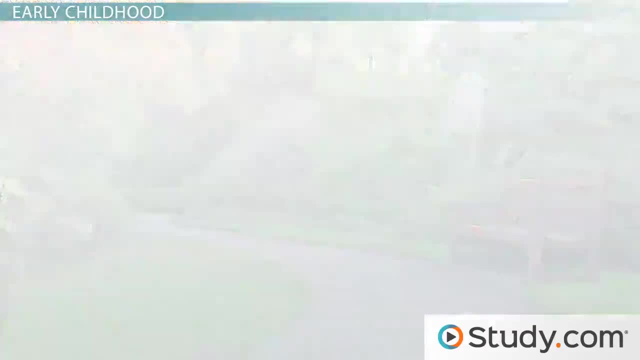 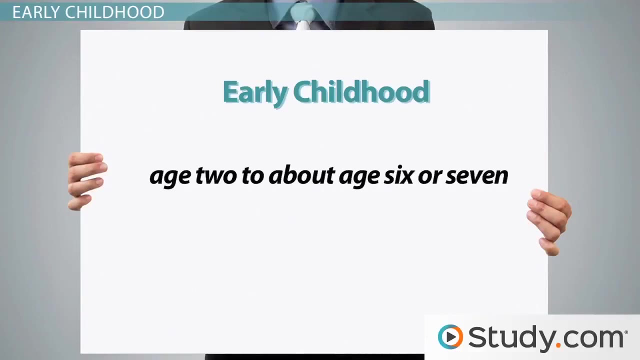 involves moving from one phase of life into another. Early childhood is the time from age two to about age six or seven. It's different from infancy in several ways. As a baby, for example, Lainey couldn't do much exploring. She would just lie around and didn't go anywhere. 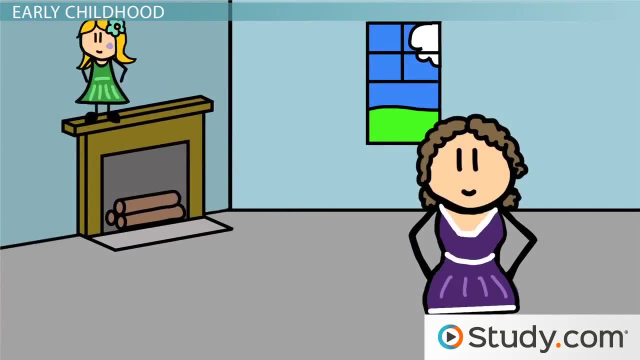 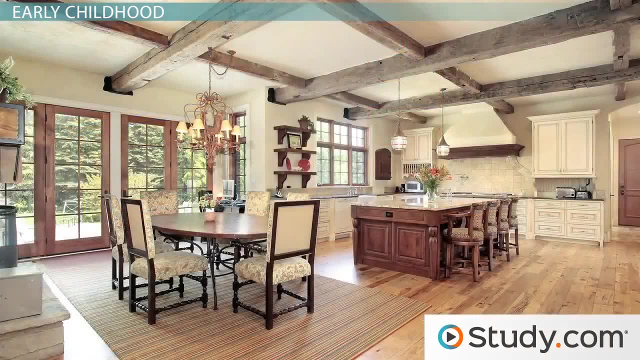 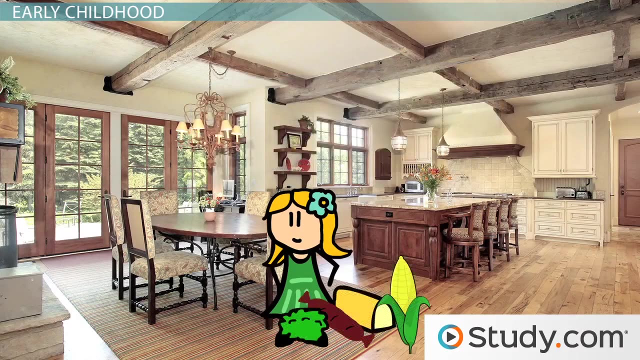 Now, though, Lainey is into everything. Ellen has to watch her very closely to make sure that Lainey doesn't get into trouble or get injured. Lainey has changed in other ways too. She can talk now, whereas before she could only cry or coo. She eats solid foods. 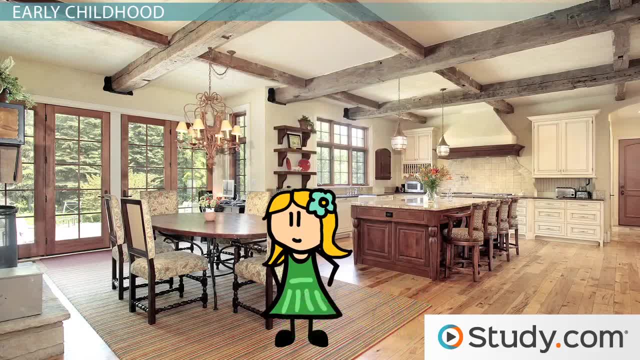 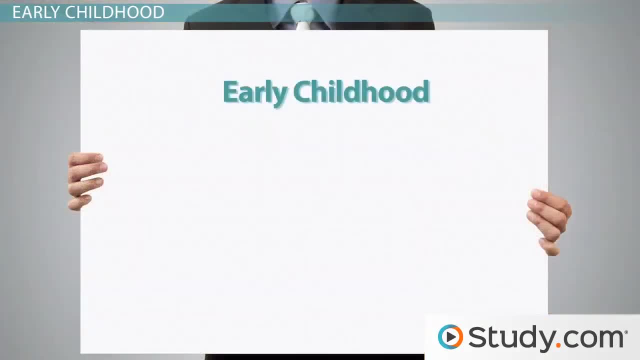 but when she was a baby, she only drank milk or formula. She's getting bigger every day and understanding more and more about the world around her. All of these changes are part of the period of life called early childhood. Let's look closer at two common concerns that 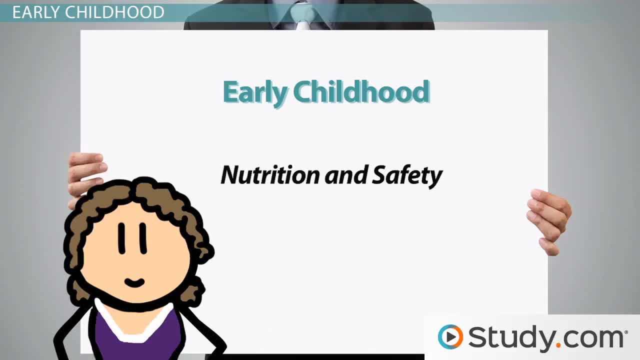 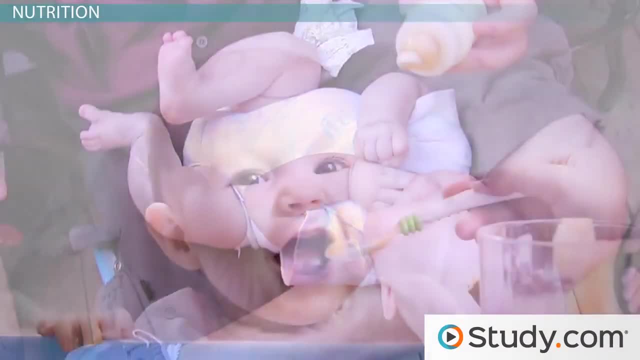 parents have when their kids are in early childhood. nutrition and safety. When Lainey was a baby, she used to eat all the time. First she would drink her bottle and then, when she started eating baby food and eventually solid food, she would drink the bottle. She would drink the. 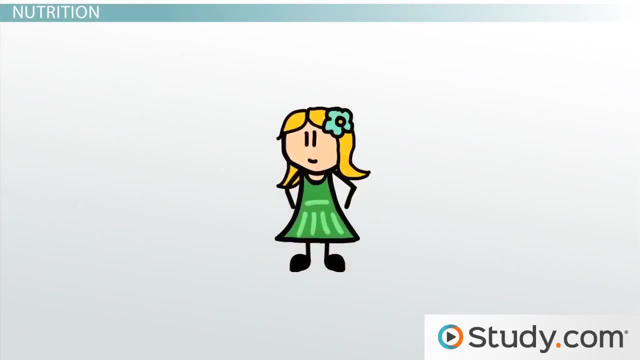 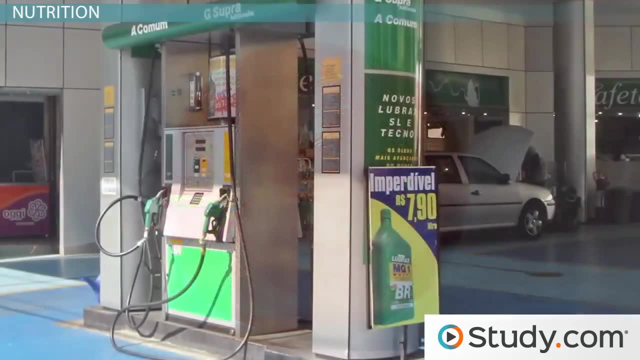 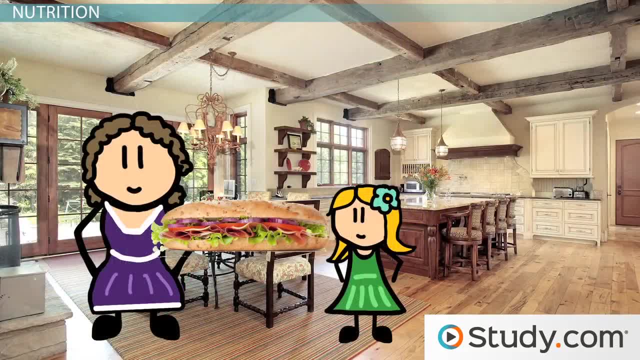 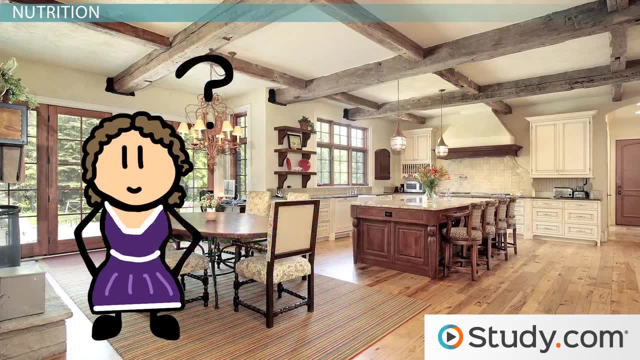 But lately Ellen has noticed a change in Lainey. She doesn't eat as much as she used to. Ellen worries that this is because something is wrong. Is Lainey sick? Is there something really wrong with her? Probably not. 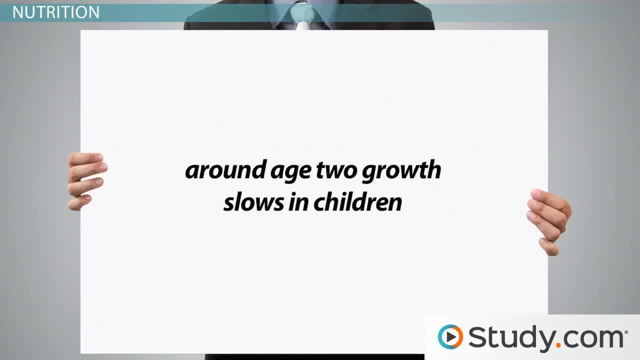 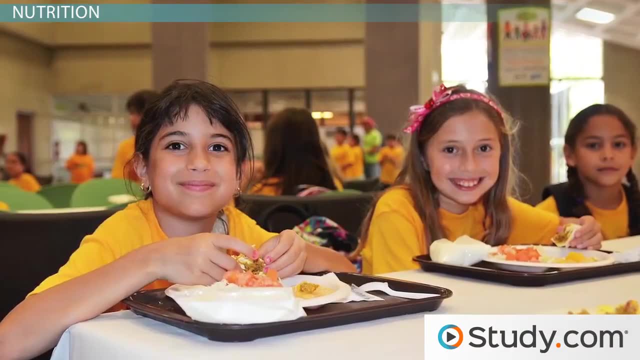 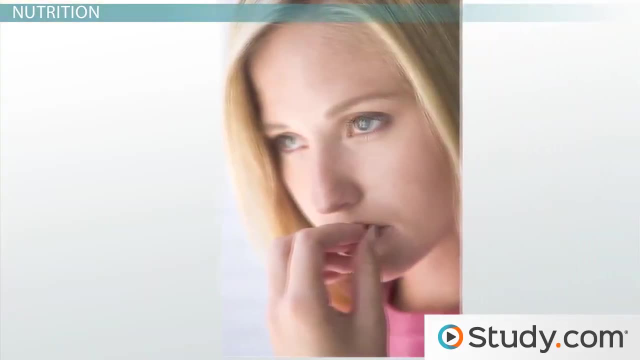 The truth is that around age two, growth slows in children. They still grow, but not as quickly as before. As a result, children don't need as much food. Most kids in early childhood naturally eat less than they did as infants. Like Ellen, many parents worry that there's something wrong when their children's eating habits change. 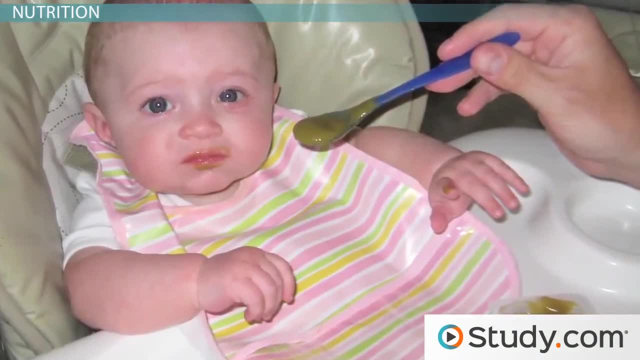 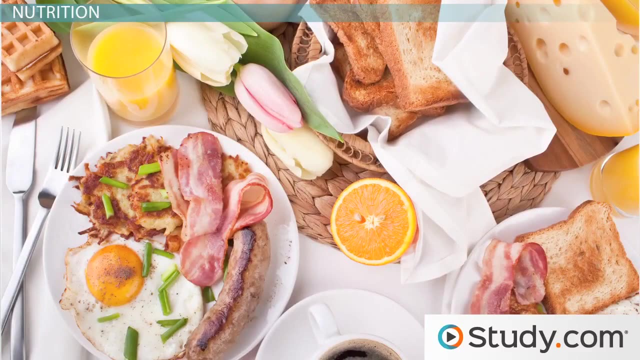 But it's completely normal for children to eat less than they did when they were babies. Forcing a child to eat more than they need is a bad idea that can contribute to the problem of childhood obesity. Another way that Ellen and parents like her can fight childbirth. 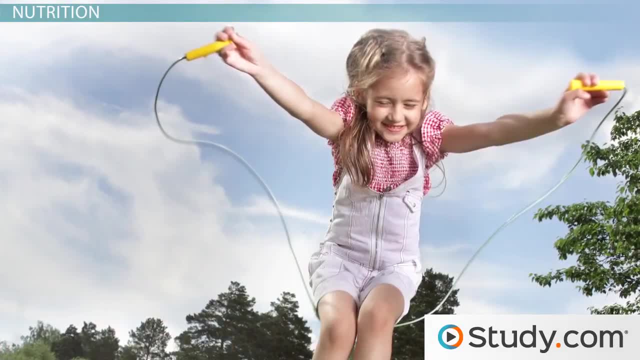 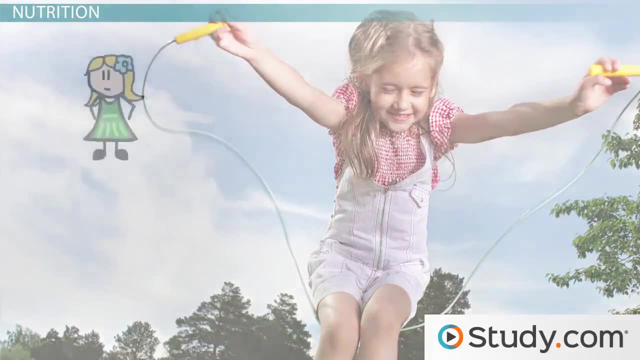 is by encouraging their children to move every day. Movement, which can be dancing, walking, running, playing or a whole host of other activities, comes naturally to young children, And parents should encourage their children to go with their instincts and move regularly. 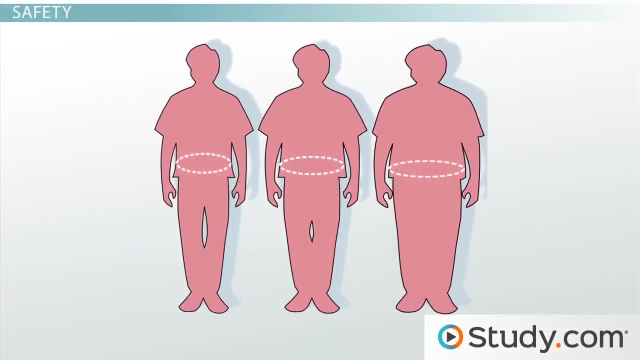 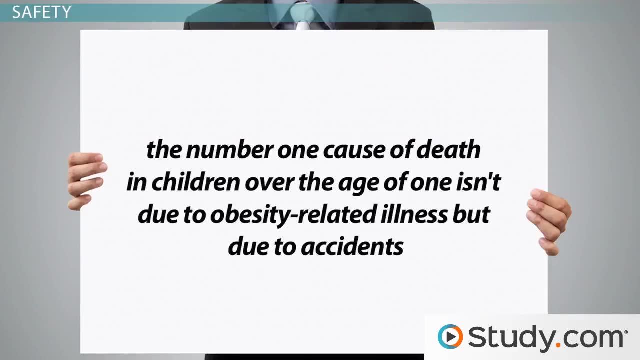 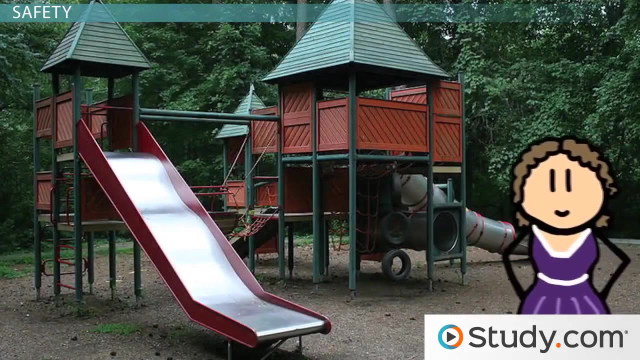 Childhood obesity is a serious health issue for many children, But many people are surprised to discover that the number one cause of death in children over the age of one isn't due to obesity-related illness, But due to accidents. Ellen knows all too well how many accidents an active and curious child can have every day. 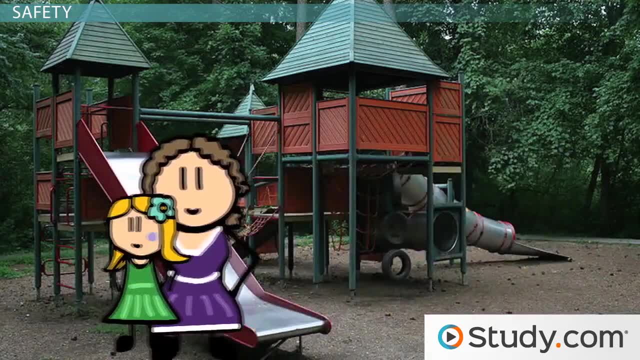 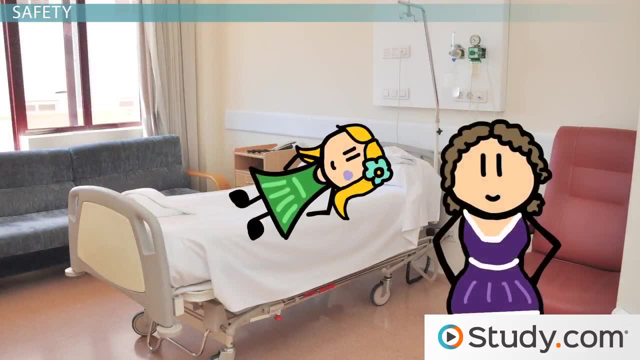 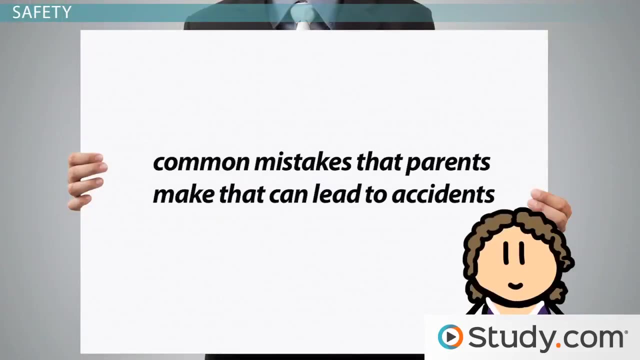 Lainey is always getting bruised or cuts. These are minor accidents and Ellen understands that sometimes they are unavoidable, But she also knows that more serious accidents can pose a problem. What can she do to protect her daughter? There are two common mistakes that parents make that can lead to accidents. 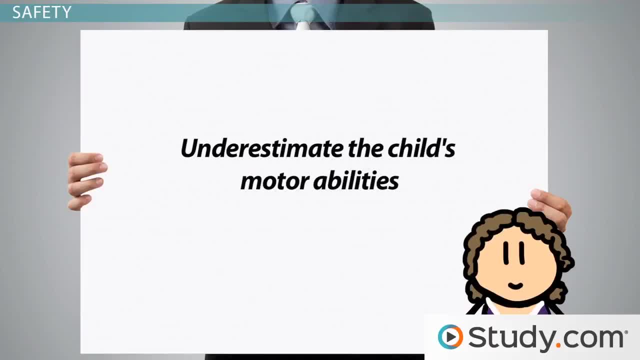 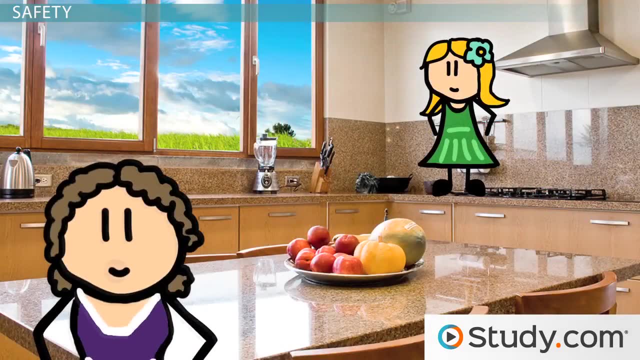 The first is that they underestimate the child's motor abilities. For example, many parents might not realize how adept their child is at climbing. Ellen was shocked one day to come into the kitchen and find that Lainey had found a way to climb all the way up onto the counter. 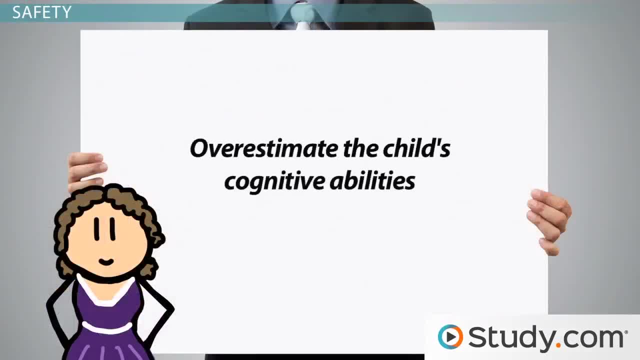 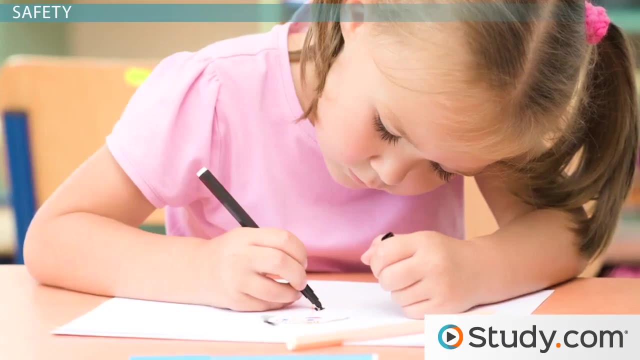 The second mistake that parents make is that they overestimate the child's cognitive abilities. Cognitive abilities are those that have to do with thinking and reasoning, And many parents assume that their children think similarly to an adult. The truth is, though, that children think, perceive and reason very differently from adults. 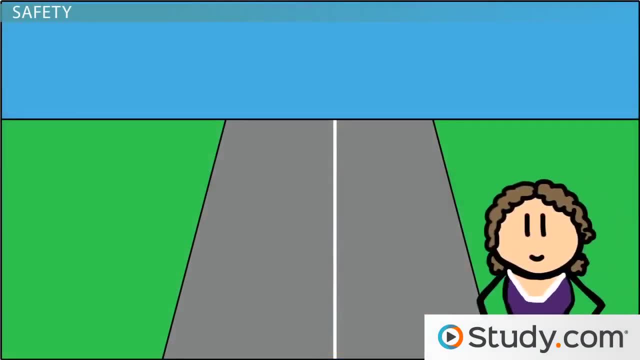 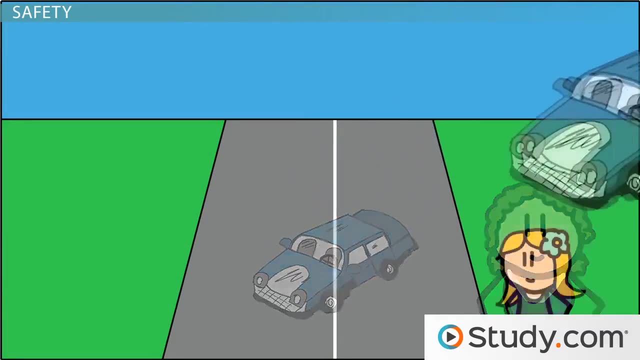 For example, a parent like Ellen might believe that a child can perceive and understand that a car coming down the road is coming quickly and can't stop on a dime. In reality, though, a child like Lainey might not understand how quickly cars move. 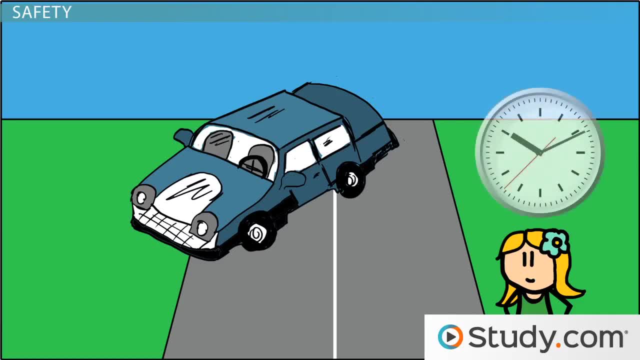 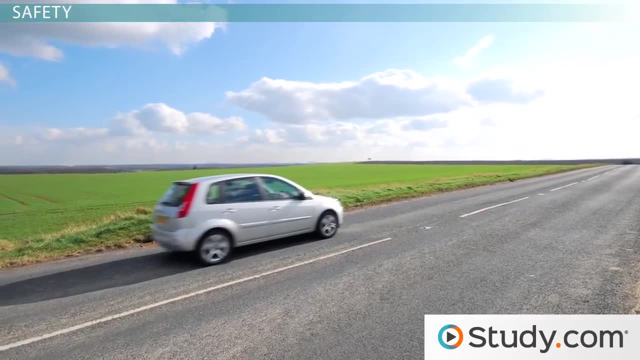 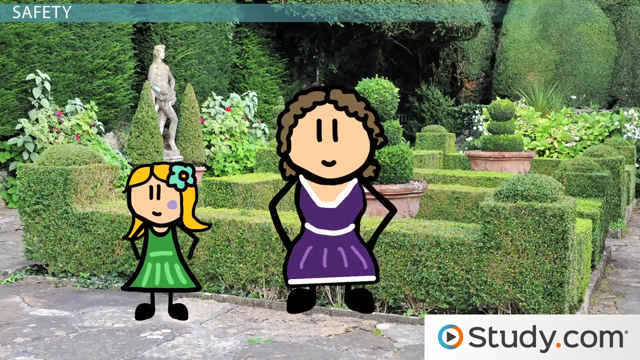 She might understand that a car can move and that a car can stop, But not that it takes time and distance for a car to stop. As a result, she doesn't understand the danger of walking out in front of a moving car. By focusing on not underestimating Lainey's motor abilities and overestimating her cognitive abilities, Ellen can take steps to ensure Lainey's safety.